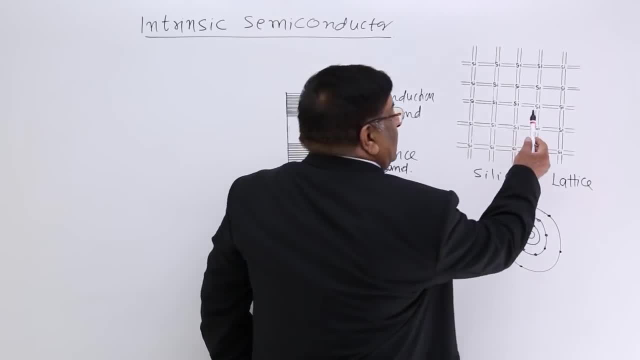 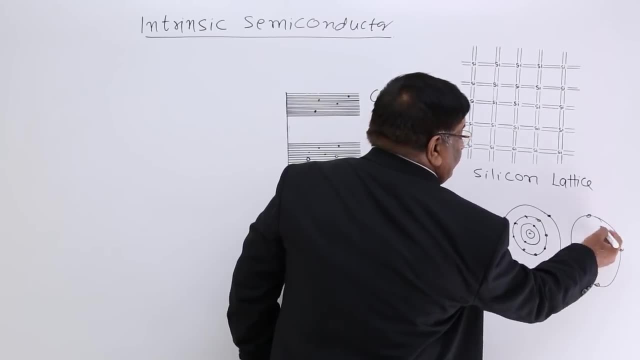 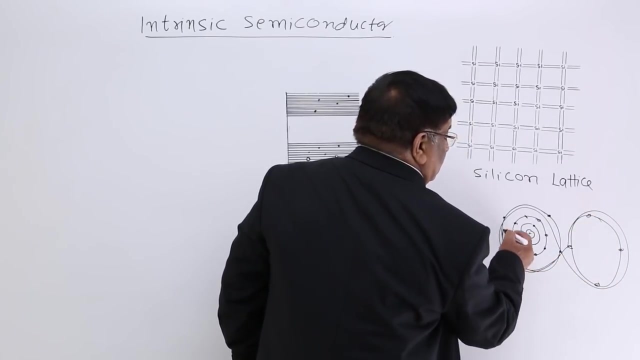 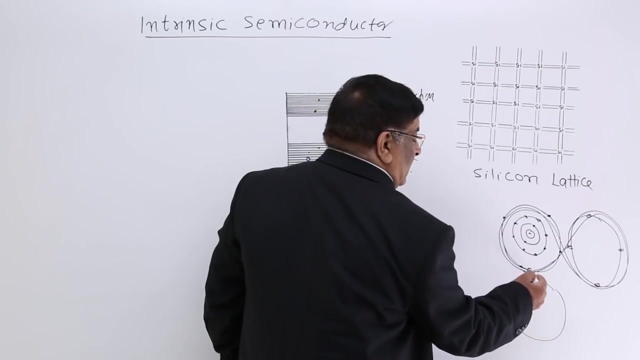 electrons. So this silicon with the neighbouring silicon, it shares 1 electron which moves like this and this electron, this moves like this. So there is a pair of sharing between the 2 electrons and therefore this one is extra, similarly one is extra from here, and there is a sharing. one is sharing with this atom and one is sharing. 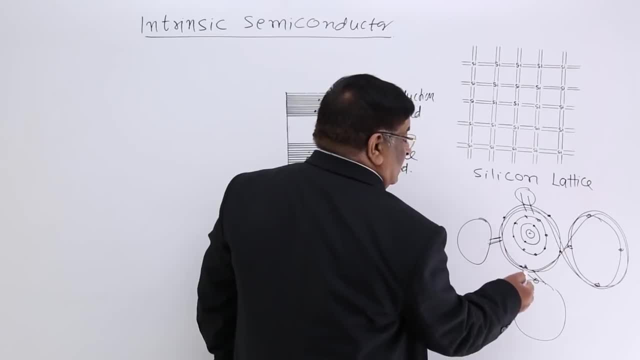 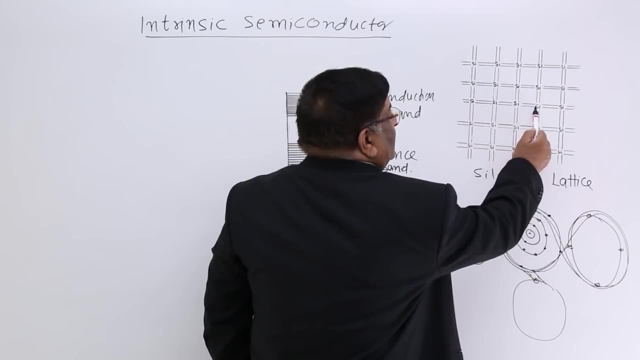 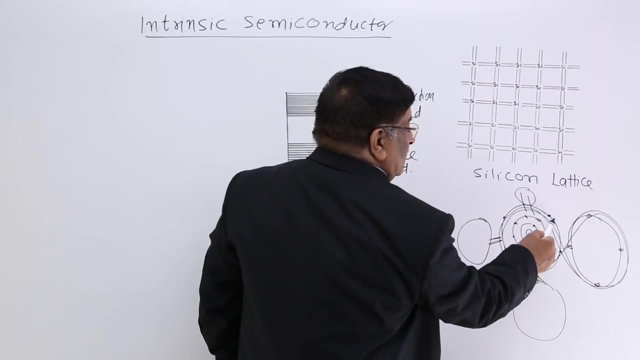 with this atom. so this double bond, this gives the indication of sharing and that is what I have made here. this silicon and this silicon, this is sharing, pair bonding, and this everywhere. one electron from here exchange, one electron exchange, one electron exchange and one change. so now this has got 4 its own and 4 one each given by all these 4, so total are 8. similarly, 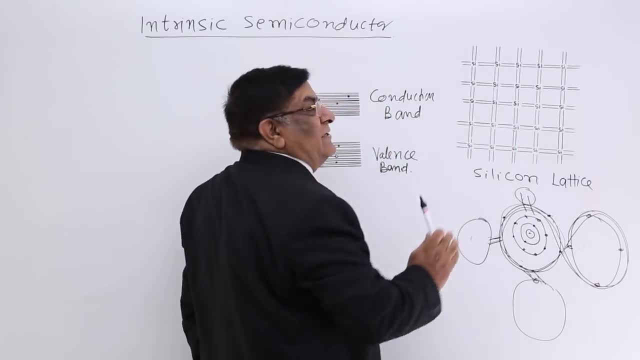 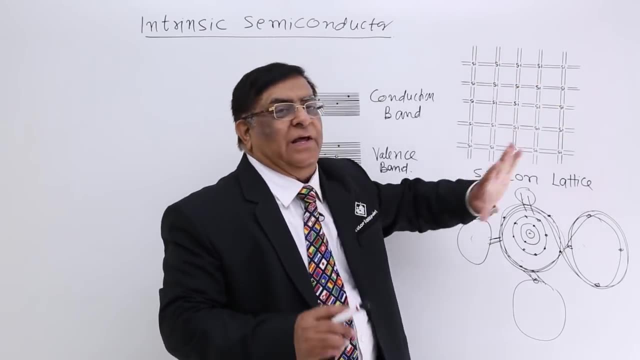 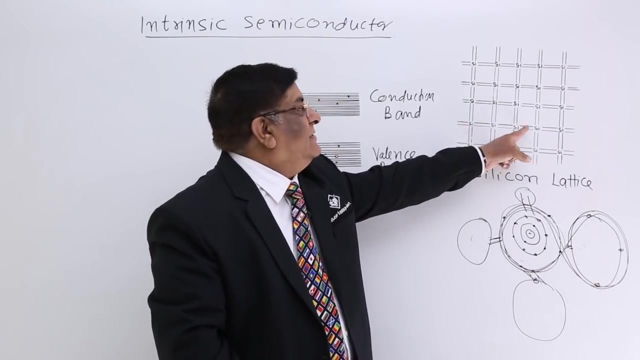 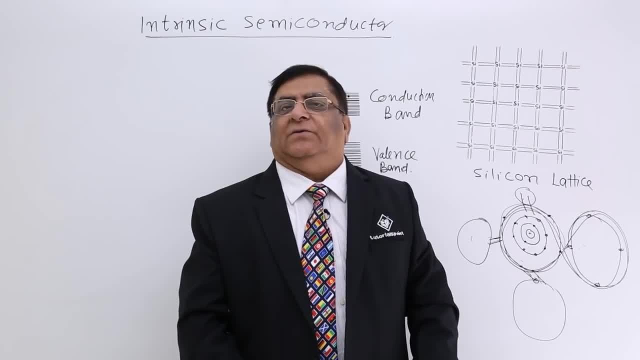 this. there may be 100s of 1000s of silicon atoms. when silicon crystal is made, we make it from the available ore In the next slide. So this is the process of purification. Now we have seen that the ore is purified and all other impurities other than silicon. 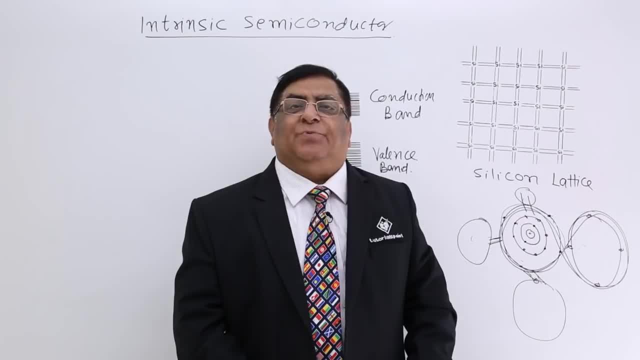 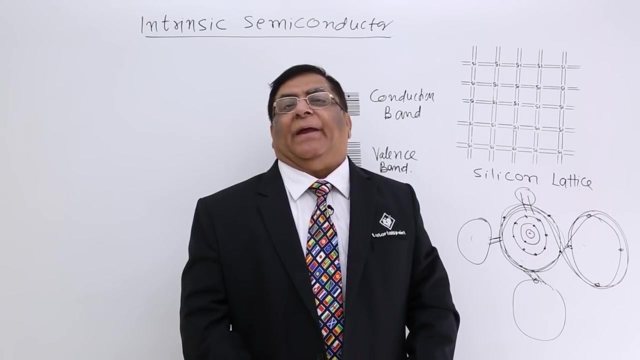 all separated out. this is the process of purification. Now we go on purifying and it is a very difficult process to make anything 100 percent pure. not a single other atom should remain and it is a big process. but there is a process in the process and if it is made, if it is done, then we get a crystal which has got 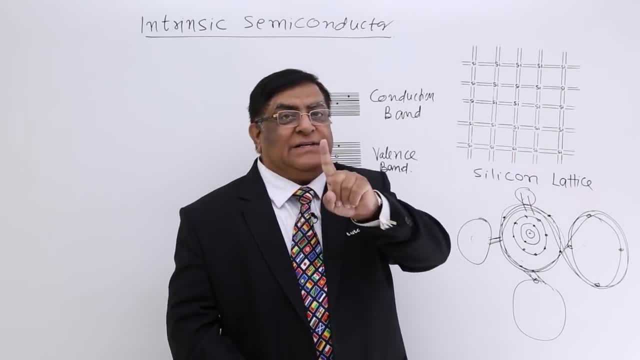 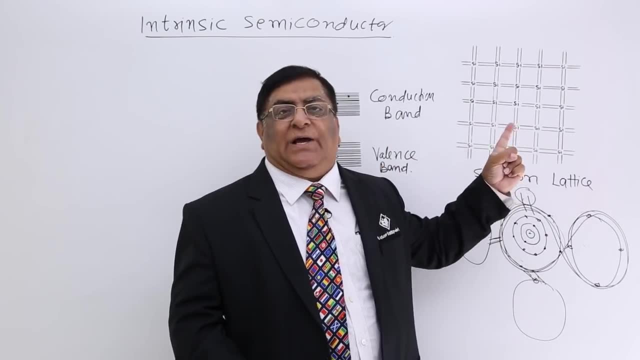 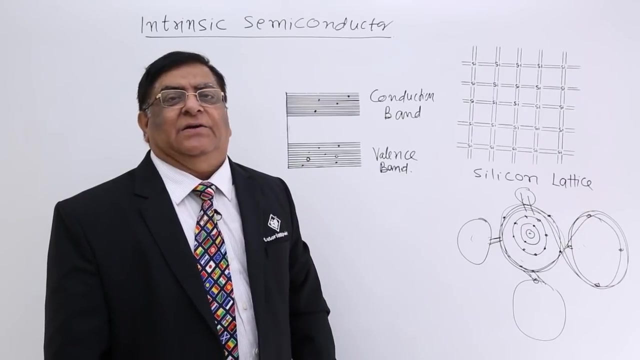 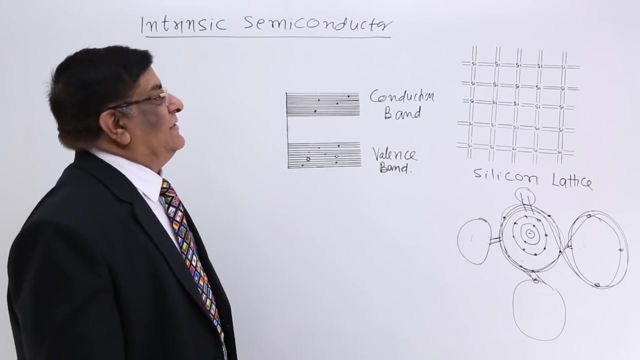 all the atoms of silicon. not a single atom is other than silicon. then this pure crystal is known as intrinsic semiconductor. so intrinsic semiconductor is the one which has got all the atoms of the same nature. That is intrinsic semiconductor. so I will write it for you see, this is intrinsic semiconductor. 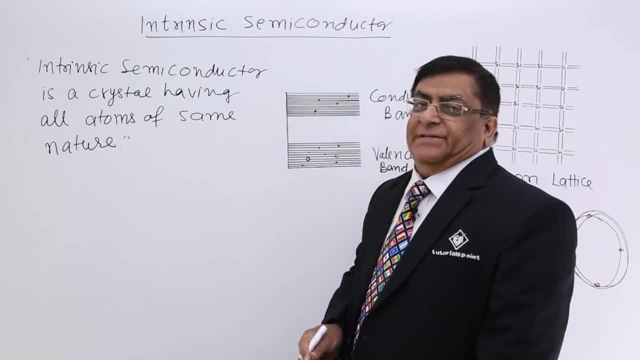 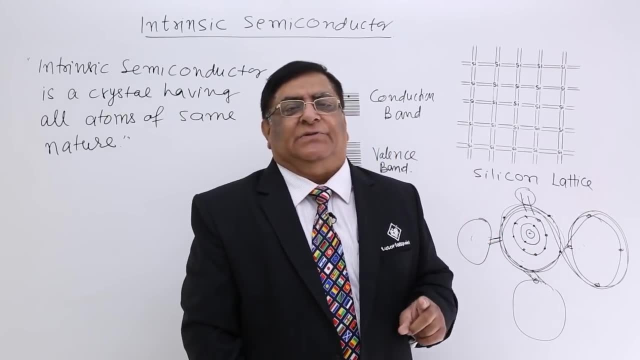 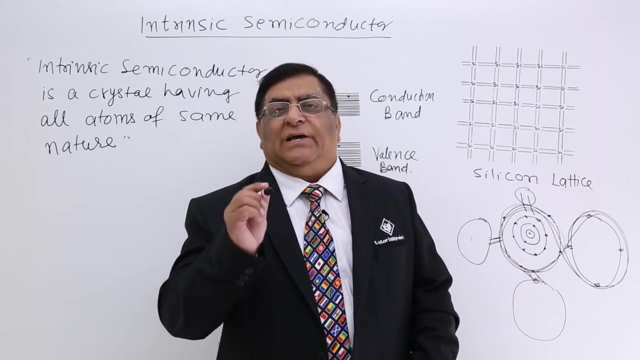 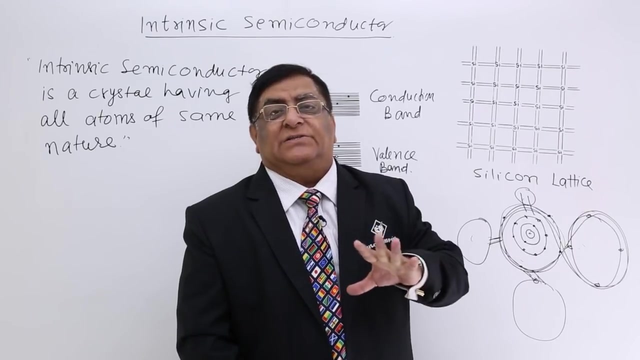 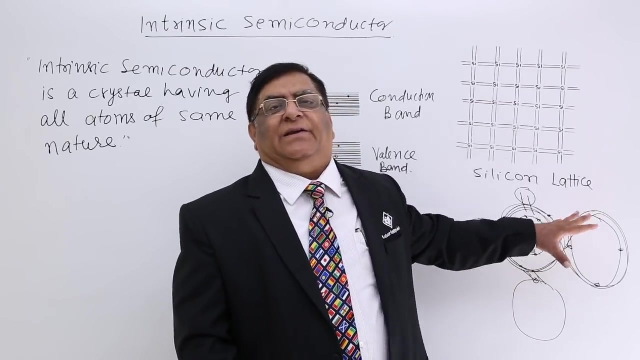 is a crystal having all atoms of the same nature. Now, what happens inside this? we will discuss it with reference to temperature. at the very cold temperature that is, 0 Kelvin, all the electrons here, all the electrons, have very less energy And that energy is just sufficient to fulfill its valence duty so that it remain a crystal. 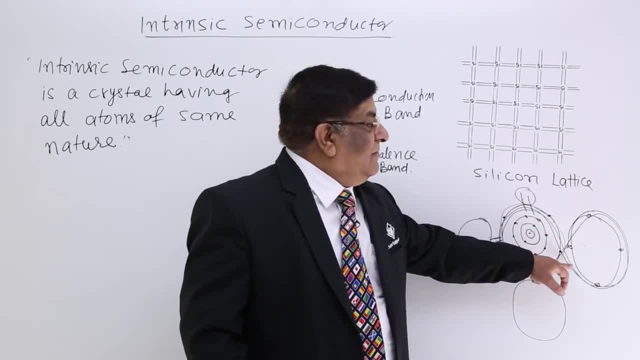 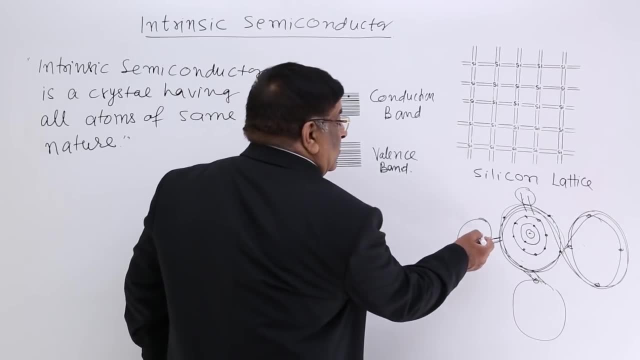 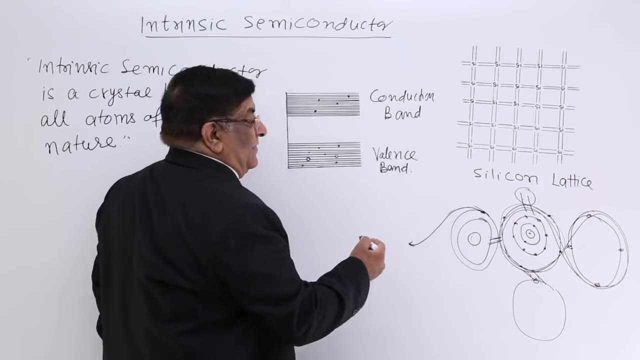 so electrons are having this much energy that they will make the valence band, but they do not have energy so that they can leave the atom and go out. they cannot leave the atom because this will need a higher amount of energy and they do not have. 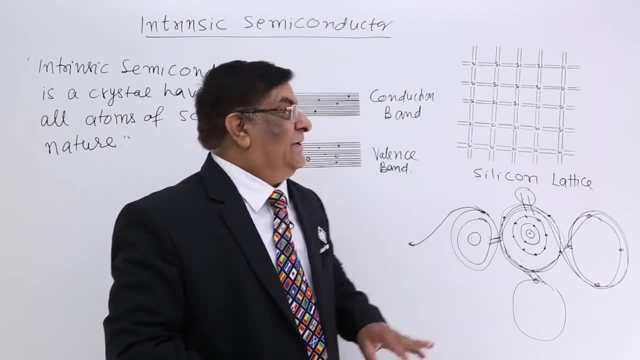 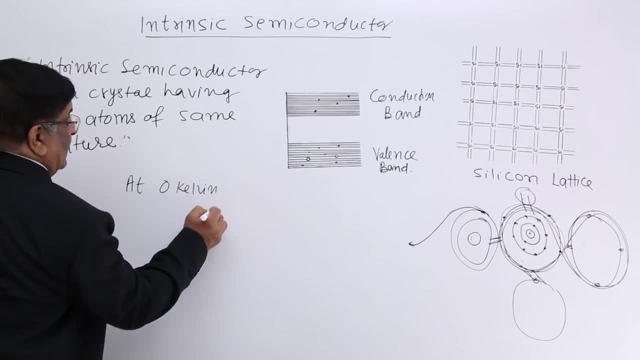 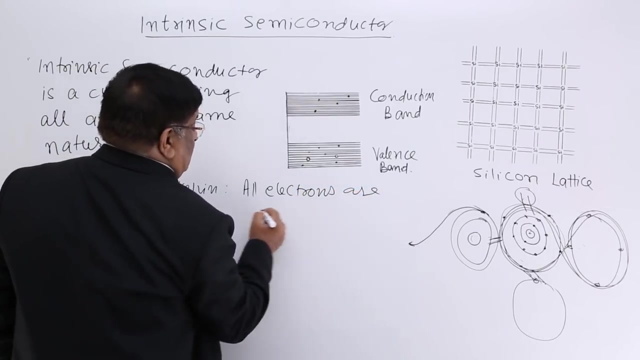 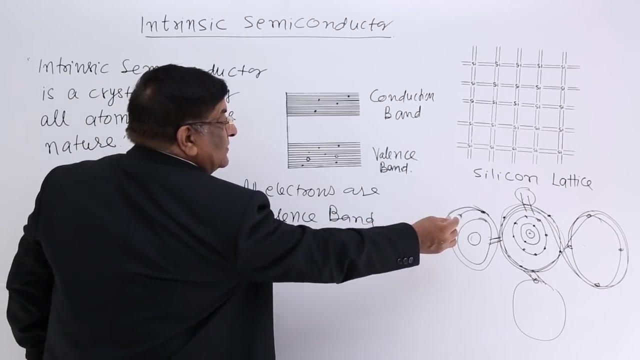 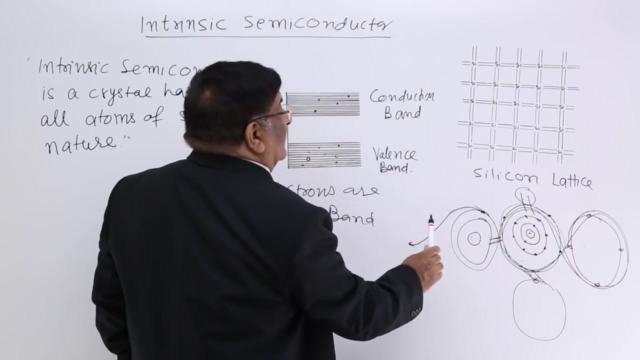 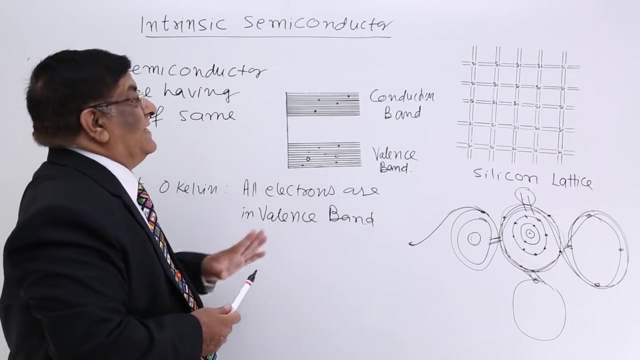 Where, at low temperature, at 0 Kelvin, all electrons are in valence band. So if all electrons, no one is free, all are having that much energy which can do on its own, Then in the language of the graph, energy graph, what we will say: all electrons are in valence. 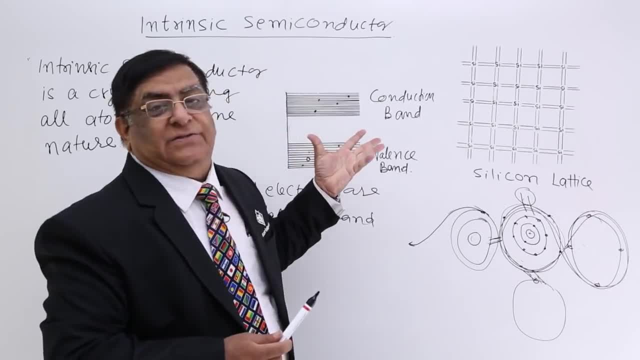 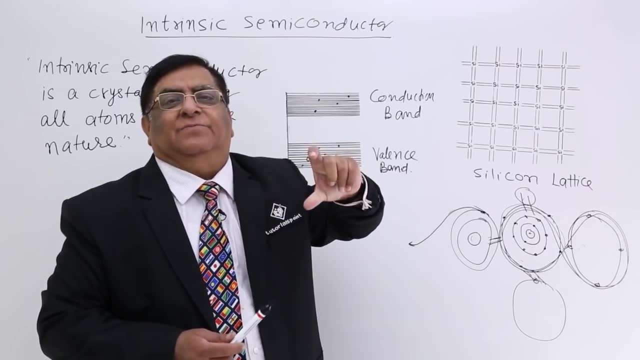 band, that does not mean they have left this place and gone somewhere else. they are here only in the atom and they are rotating. When we say they are in the valence band, that means when we make a graph, then we have to show them in the valence band. So valence band.